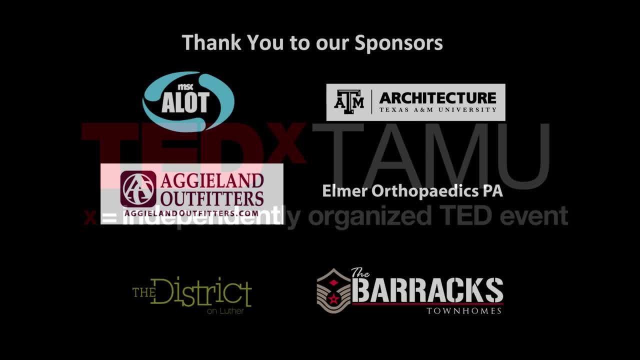 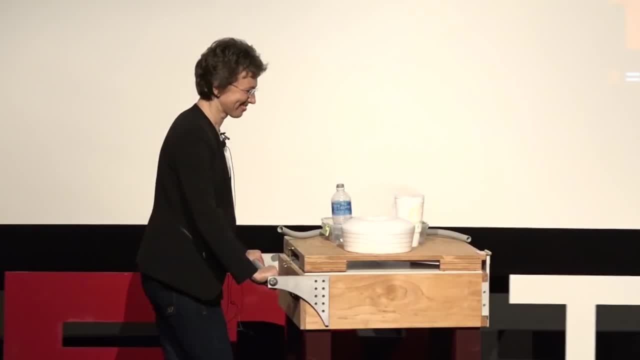 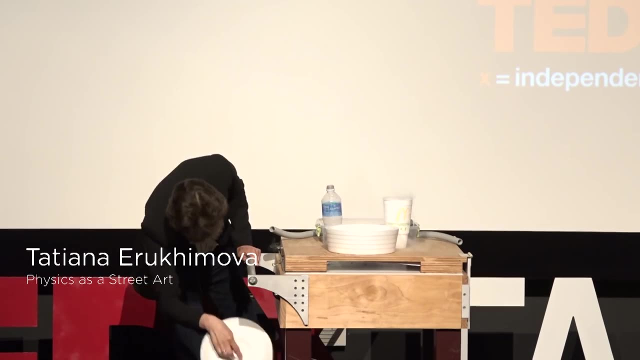 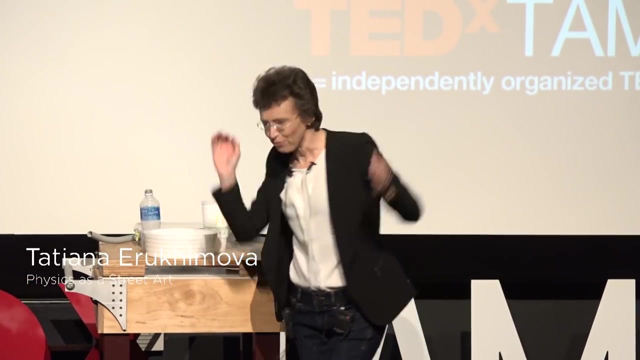 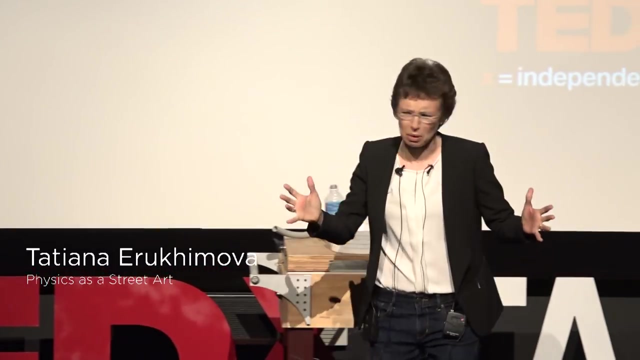 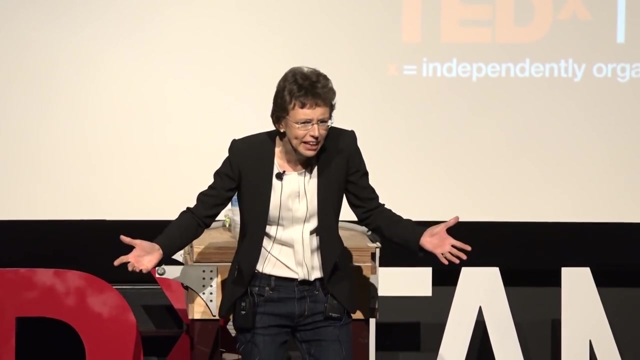 Before I even start, I have to share with you my secret. Actually, I already did. I opened my mouth, so you know that I didn't graduate from a high school in Texas, And yet I teach And I communicate science And I communicate physics. What could be worse? 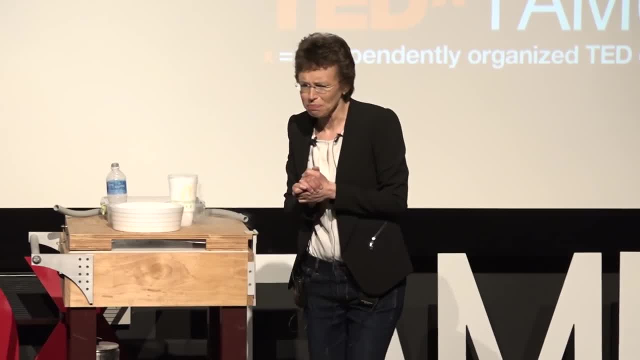 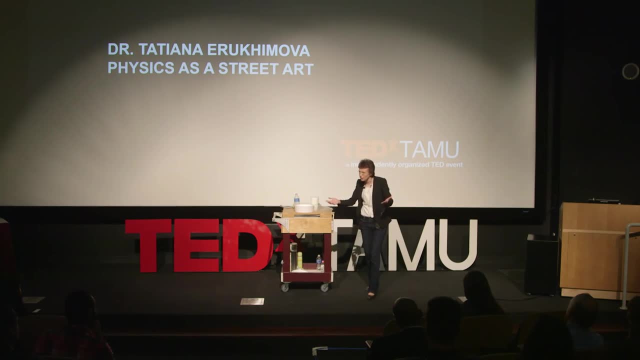 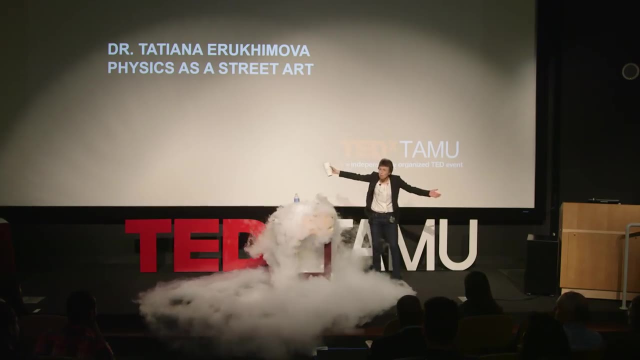 So I need all your help today. You know I do physics shows Children. schools come and I show them experiments. They're children, so I have to impress them to keep their attention. Something like this: I dropped liquid nitrogen, basically liquefied air, crazy cold liquid and moist cheese condensed. 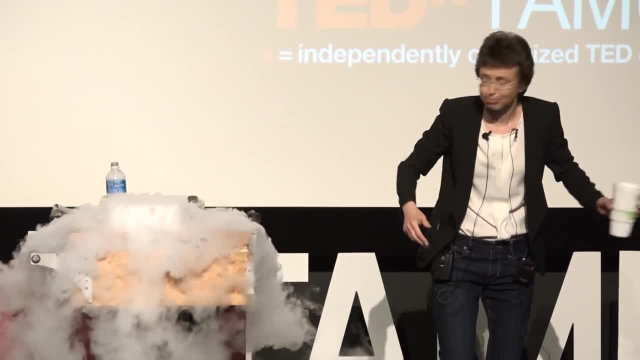 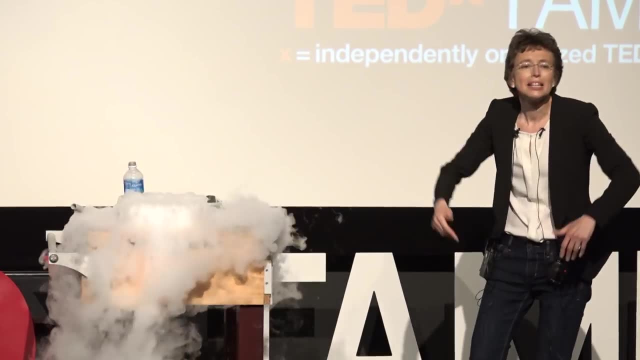 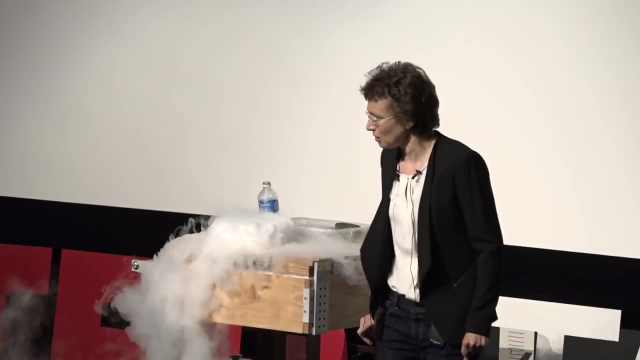 We made a cloud. I like clouds. Who doesn't? If children were here in this room, they would start screaming: do it again, do it again. Children are scientists. I remember once I did a physics show and the little guy came to me and said: I know your secret, You're. 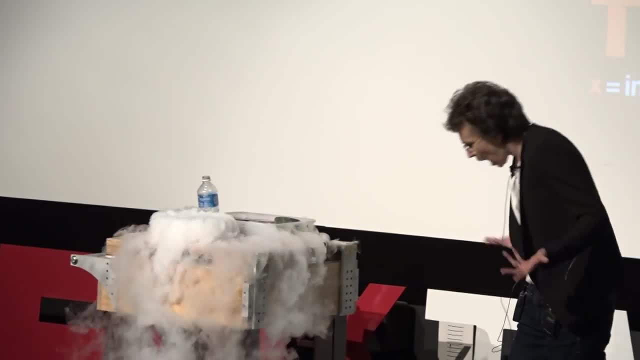 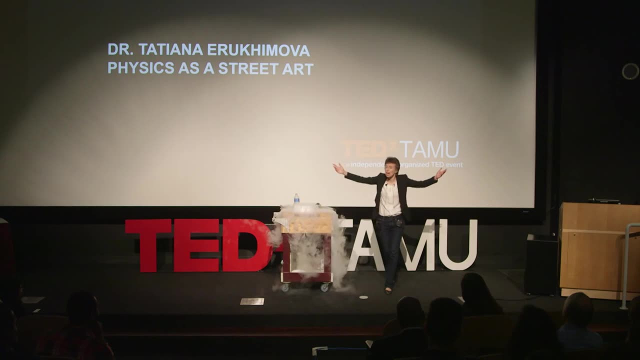 not from Texas. I asked: how do you know? And he said: you have a British accent. How flattering was that. How many of you would think that I have a British accent Once it was even more interesting. We went skiing, And when you ski, you take a lift. 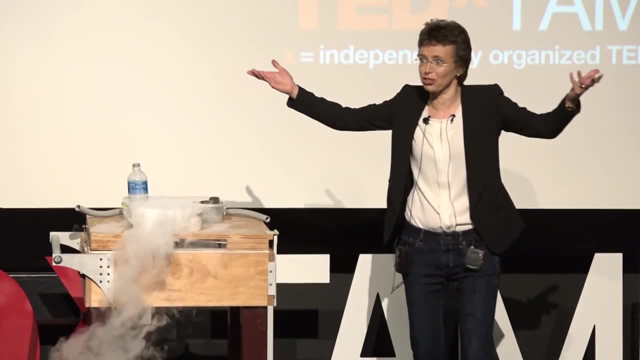 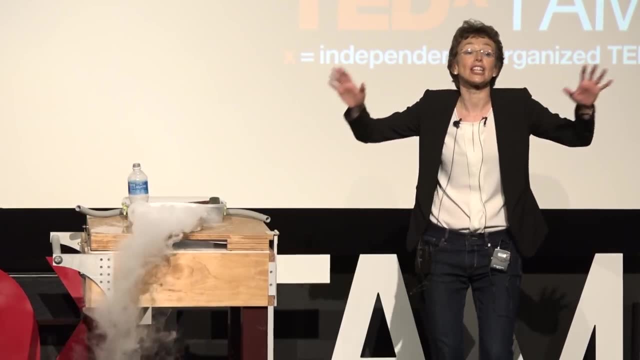 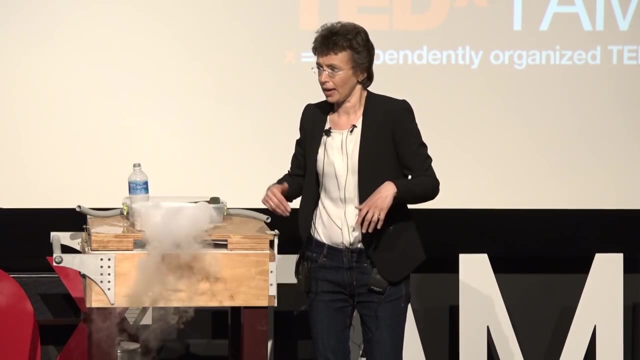 to go to the top of the mountain. You're up in the air with strangers, so you don't discuss anything controversial like gun control or climate change. No, All conversations are just exchange of pleasantries. So there was a lady next to me and she said hi. And I said hi And she said: are you? 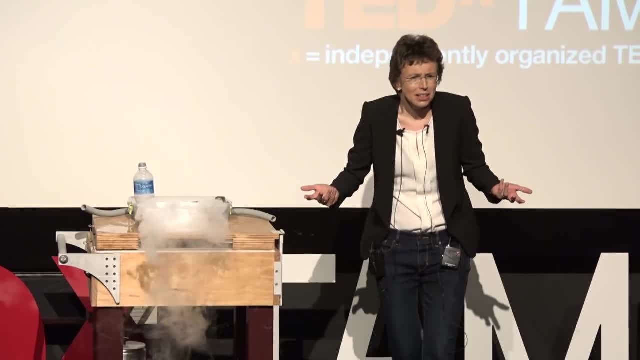 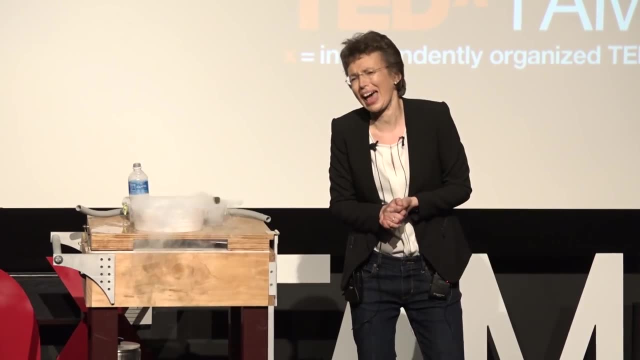 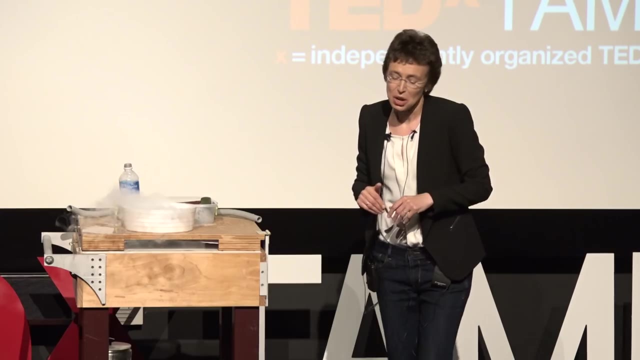 from Russia. Is it that bad? I just say hi and you already know that I'm from Russia. And she said: relax, I'm a speech therapist. Once I had life-threatening experience. while I was riding this ski lift, A guy was sitting. 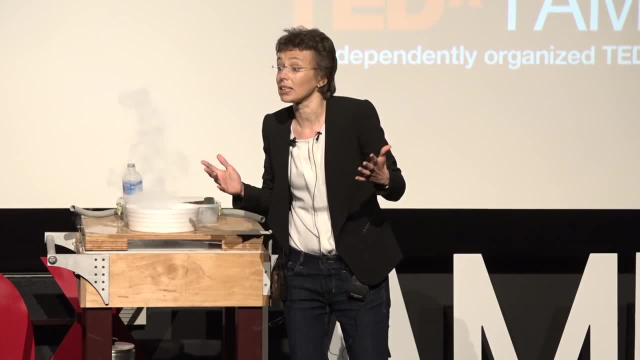 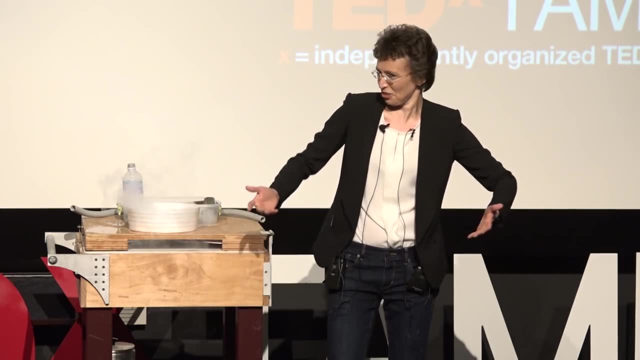 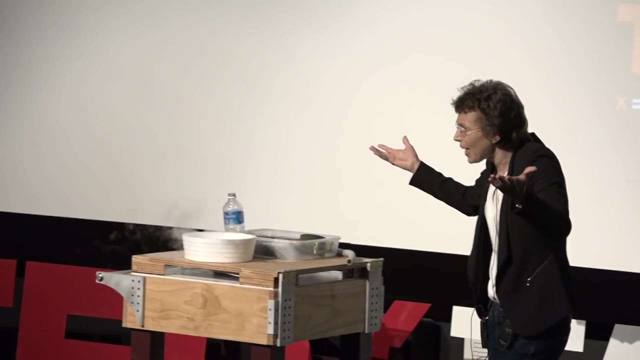 next to me. I opened my mouth, so he immediately asked: what brought me to US? I said job. What do you do? I teach. What do you teach? I said physics. He looked at me and said: get out of here. We were up in the air. What can I do? We ended up that 10-minute trip. 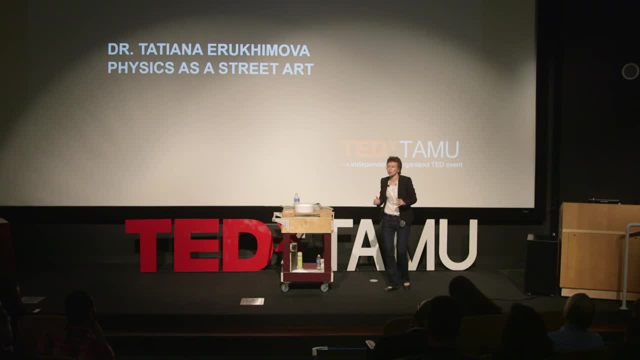 as friends, probably because of a single reason: I didn't waste my time and I invited him to our festival. And here the story begins. Just last weekend, we had an amazing event here on campus: the Texas A&M Physics and Engineering Festival. More than 5,000 people came to the festival. 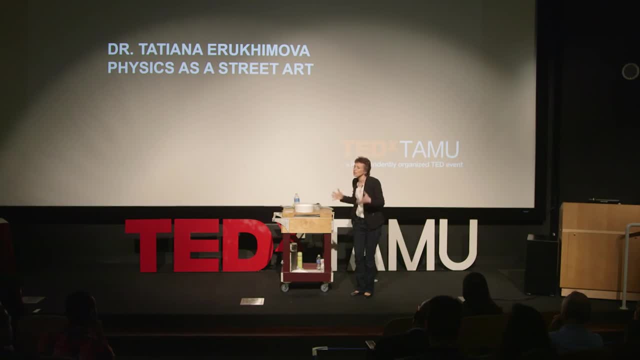 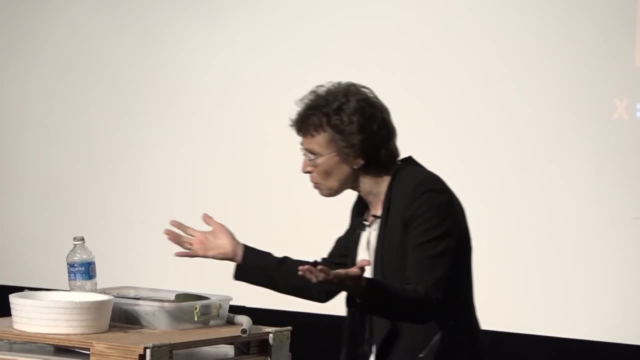 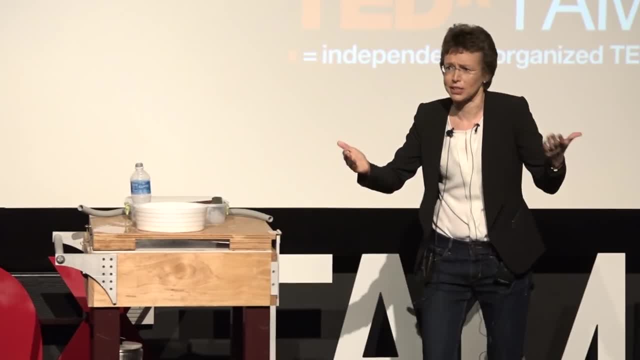 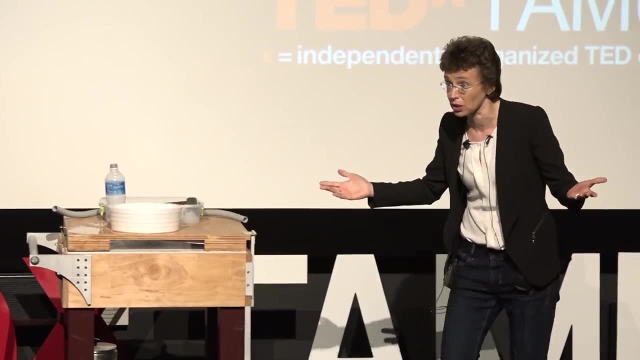 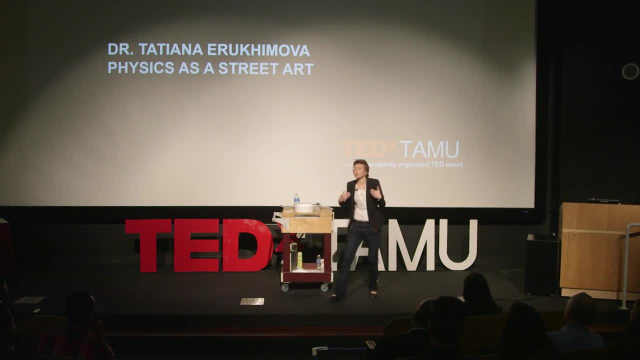 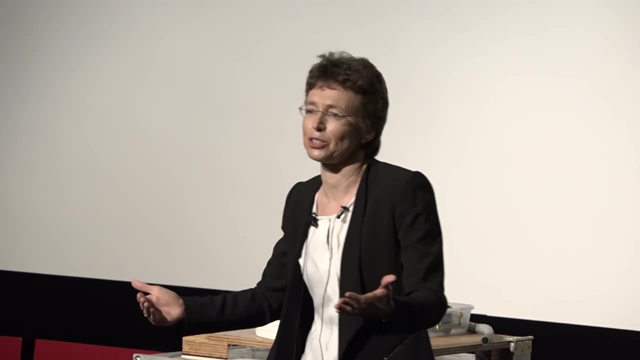 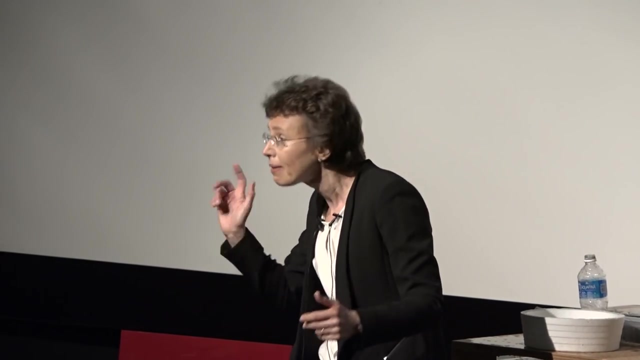 for us to celebrate wine. Why are we so surprised? Why are we so impressed that all these people came here, spent all Saturday playing with hands on demonstrations, attending talks, learning without even knowing that they were here- Yes, knowing that they were learning. Why are we so happy about that? There is a reason: Public. 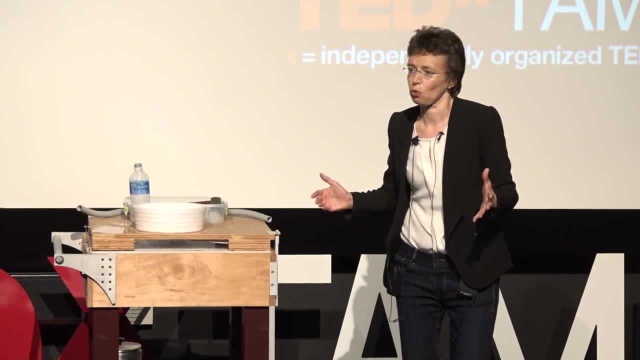 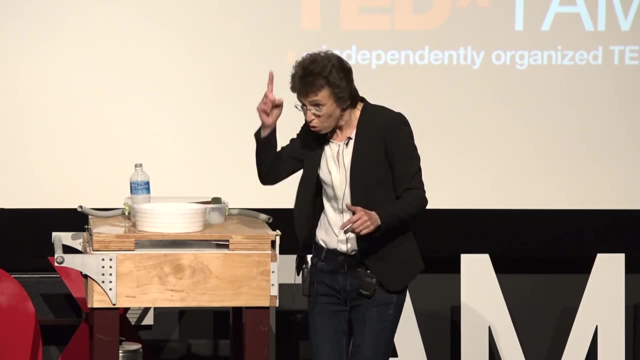 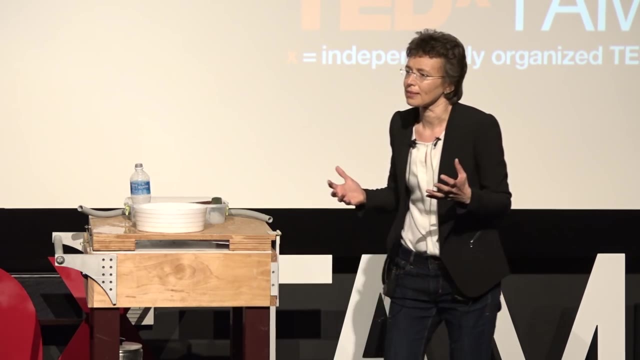 respect for science is disturbingly low. It's actually interesting how it works. If you tell somebody that you are a scientist, it is always met with respect: Oh, you must be smart. At the same time, respect for the scientific method, the results of science, is very low. 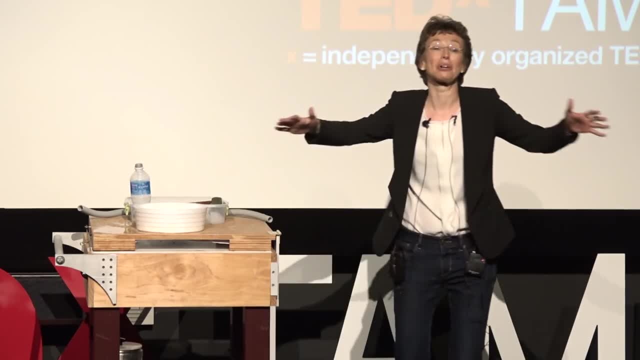 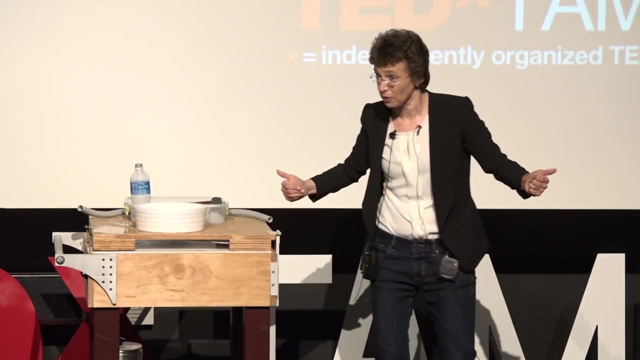 Of course, it's not that bad. I remember I did a physics show at a local elementary school. It was a big gym. Children were sitting on the floor. I was standing in front of them, I was performing the experiments. There was a five-year-old. Every time that I did an 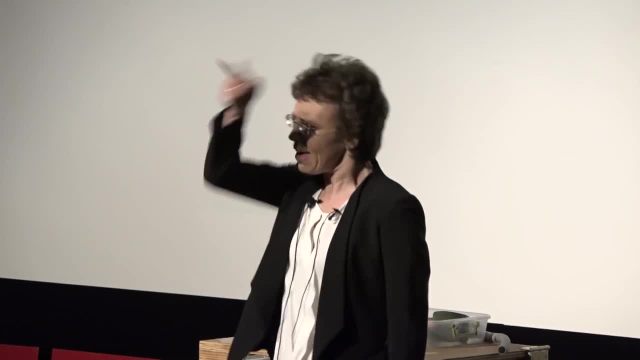 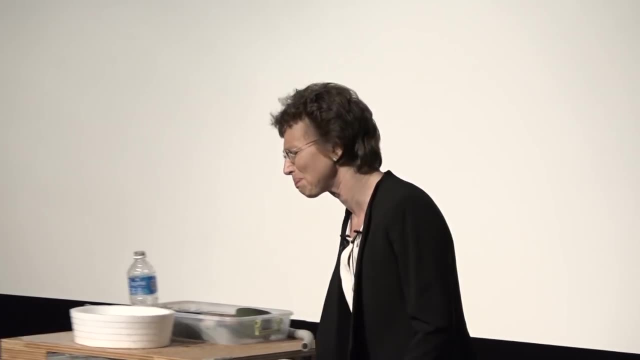 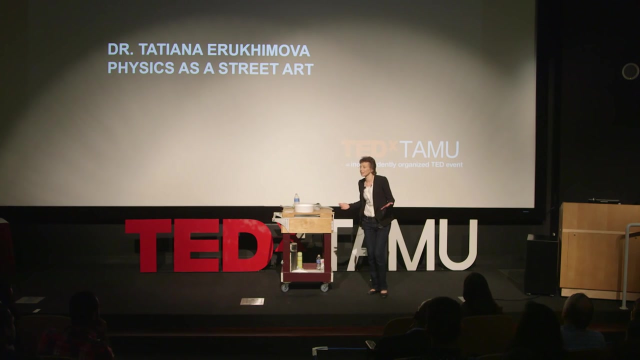 experiment, he would stand up and say: that's science. I wish everyone has the same respect for science as that five-year-old. Many people are talking about STEM disciplines, that we need more students majoring in math, science, engineering. I agree with that, but there is something even more important: Not everyone has to major. 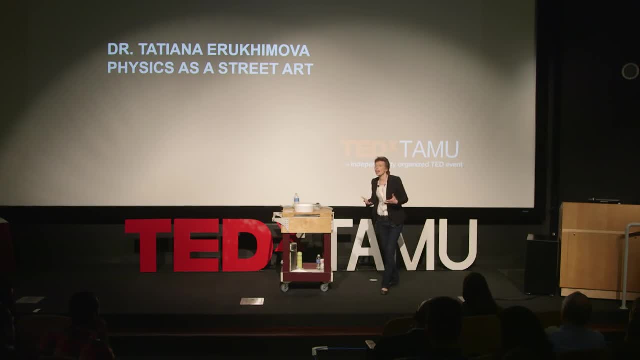 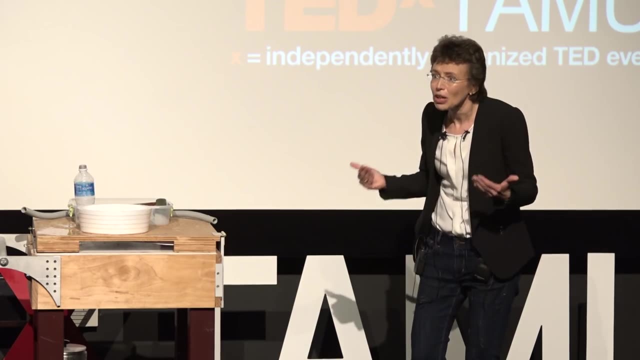 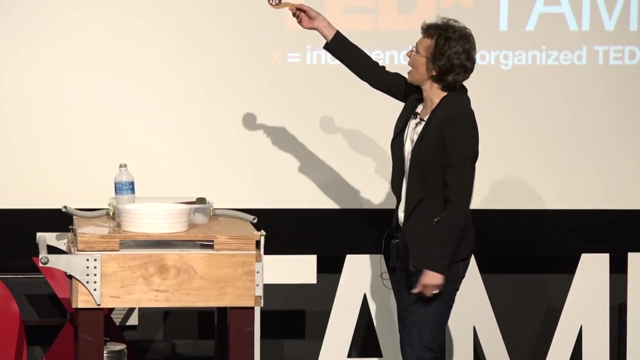 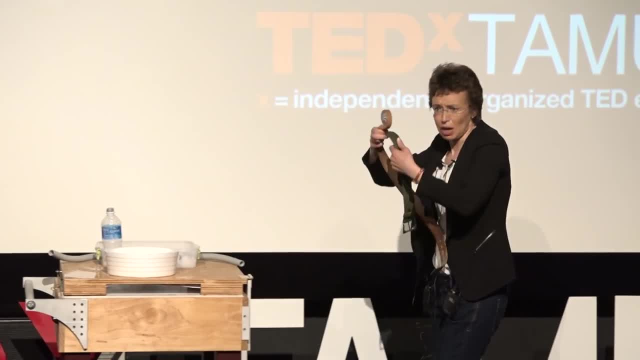 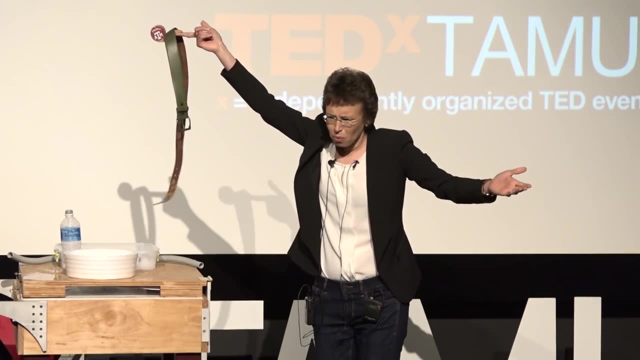 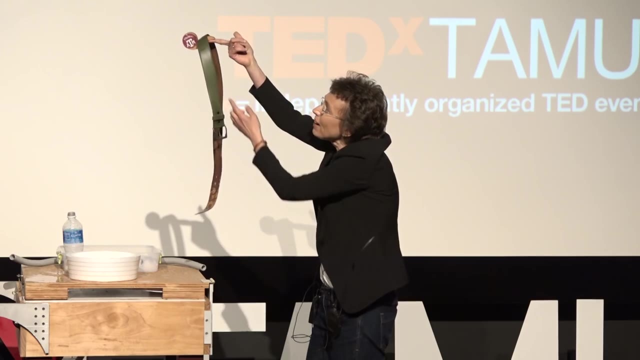 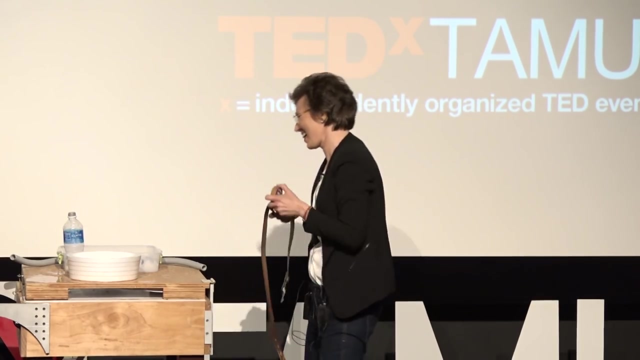 work. Now look, I make things even worse. I put a heavy belt here. Watch What's going on. Why. If you look carefully, you will see that we move the center of gravity under my finger. We balanced it. That's science. Recently I had to ride this cart to another side of. 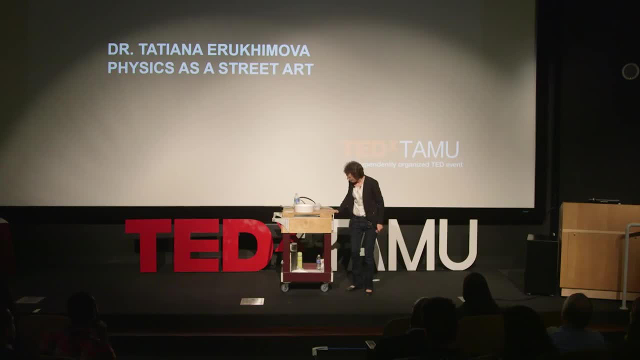 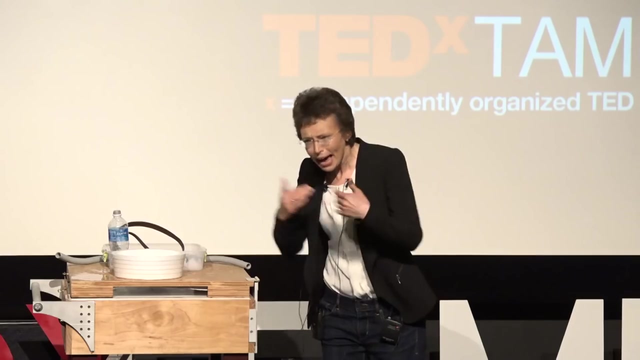 the campus to show the experiment. Thank you. This is a tall cart with heavy top, so the center of gravity is way up and the pavement on campus is uneven. You know what happened? I pushed the cart, the cart flipped over. I flipped over with the cart- liquid nitrogen. 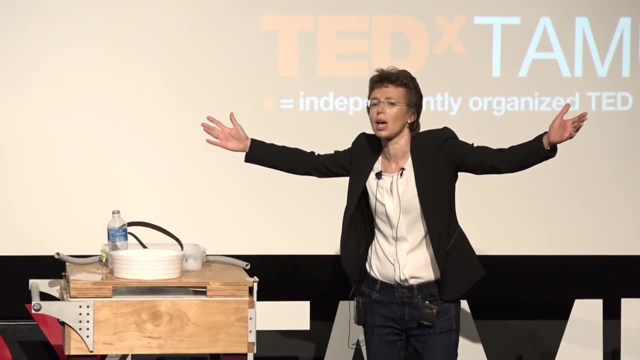 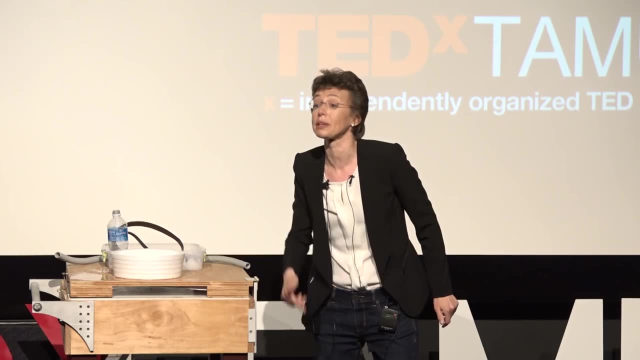 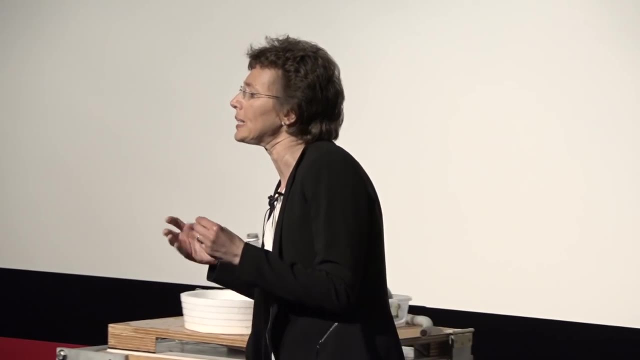 escaped my doors and made a beautiful cloud. And there I was, lying in the middle of this cloud and screaming: help me. help me Always remember where your center of gravity is. Sadly, many people consider universities as ivory towers where professors sit and do. 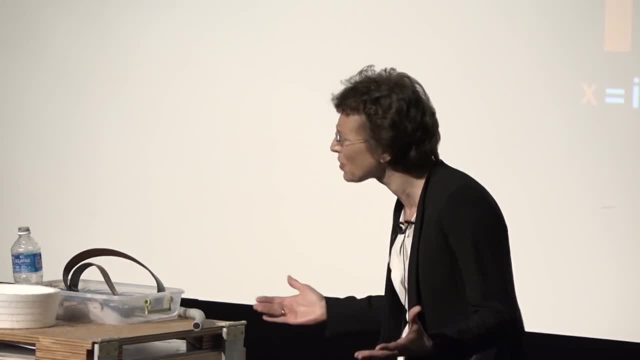 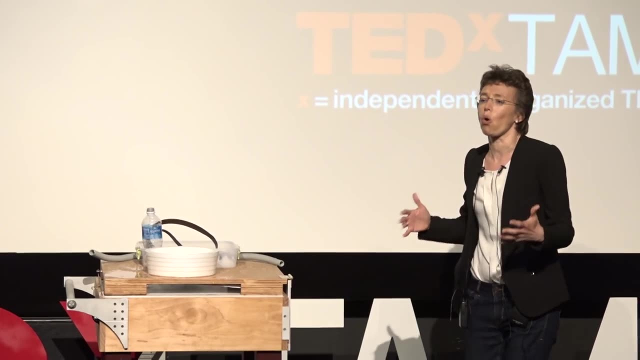 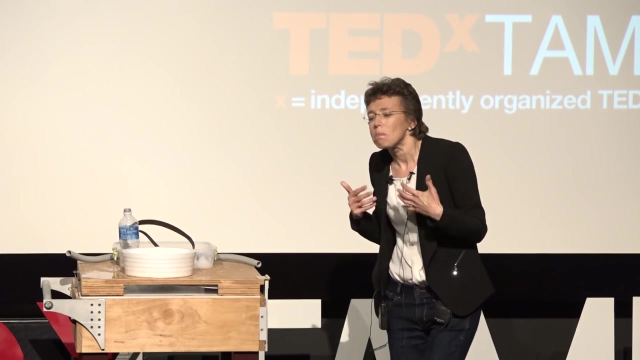 something obscure and irrelevant to the society. Of course, this is hugely unfair. All modern technological marvels- computers, the internet, telecommunications- all of them originated from basic research. How many know about that? Not many. We need to find a better way to communicate with people. 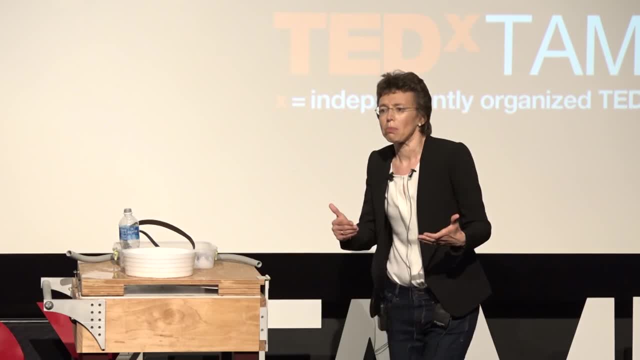 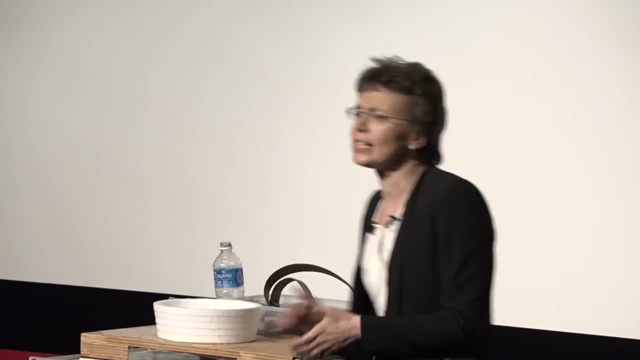 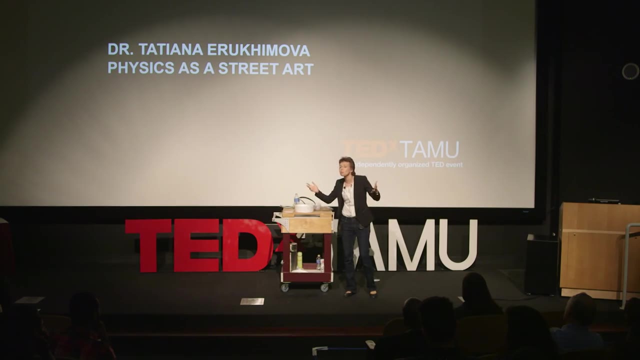 We need to rebuild the trust between the public and scientists, And here we come to science festivals again. The good news is that the number of science festivals around the country is growing. There is this amazing organization, the Science Festival Alliance, where you meet people whose 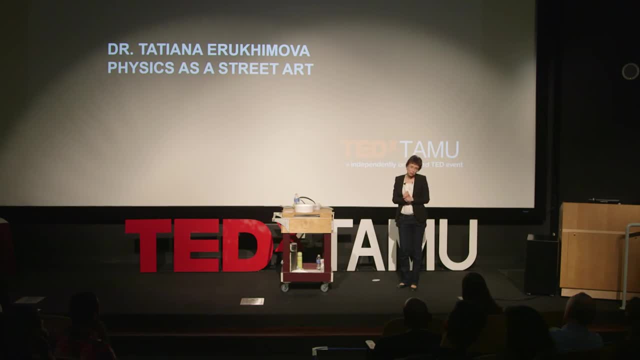 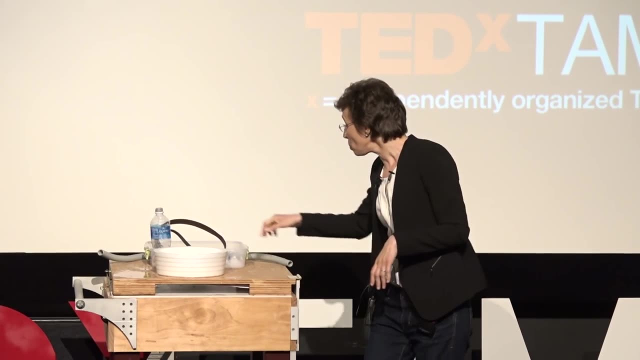 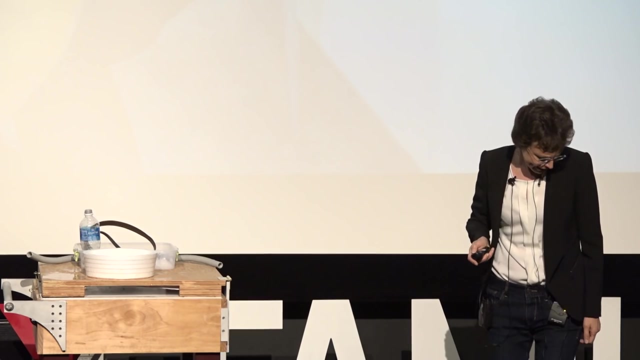 passion is organizing science festivals, But today I will tell you about my passion: the Texas A&M Physics and Engineering Festival. As always, great stories start here. The story starts with a great visionary. In the year of 2003,, Ed Frye, then head of the physics department, pioneered the change. 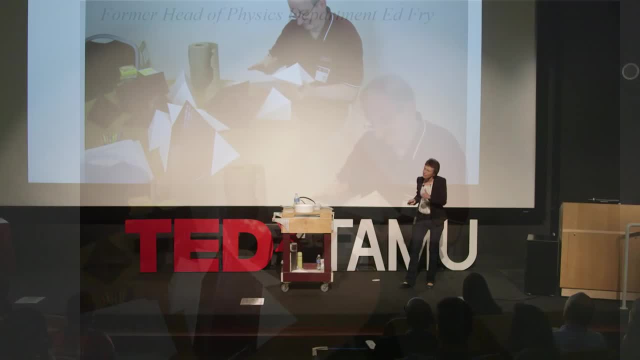 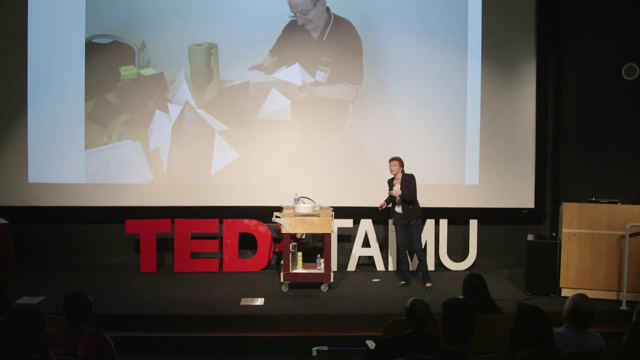 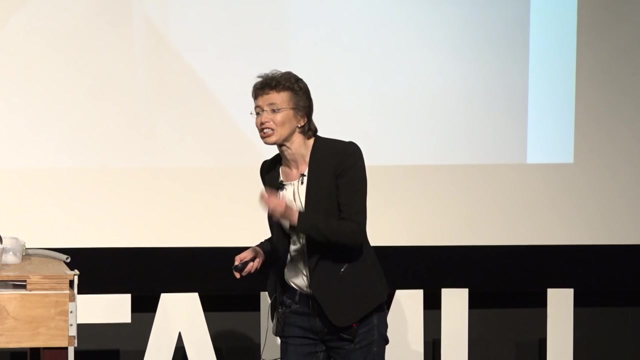 He founded the physics festival. How did he do that? In a very interesting way: he ran around the department and asked faculty physics professors to build a demo that inspired them when they were students. Since then, our festival is famous for the record number of faculty top-notch researchers. 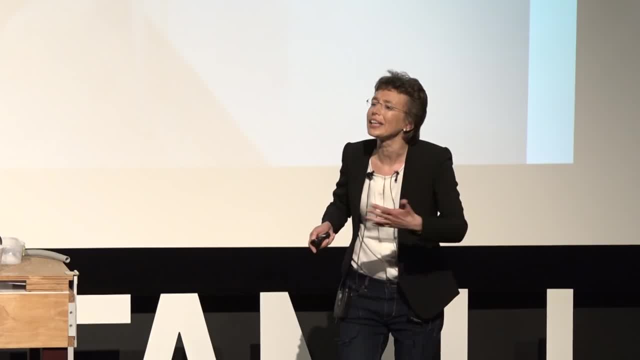 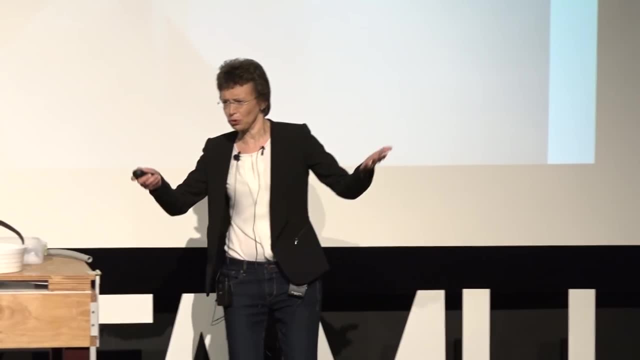 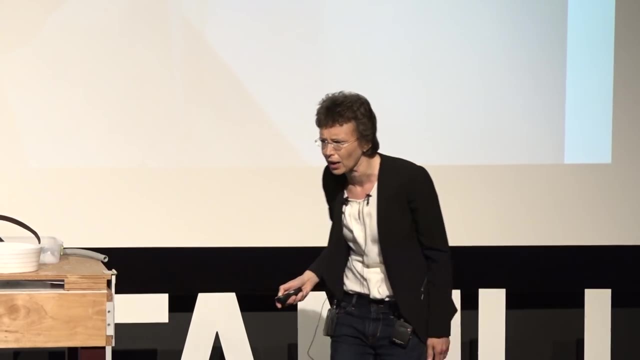 who participate in the festival, who spend all day talking to people sharing their passion for science. Let me ask you something: How many of you like to ride a bike? Yeah, quite a few. Forget about it, It's boring. We have a bike that has square wheels and still runs smooth air. 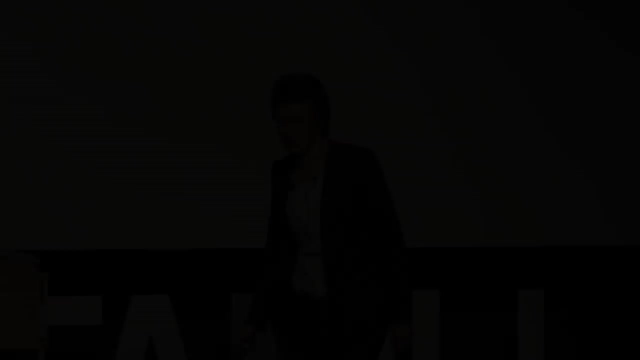 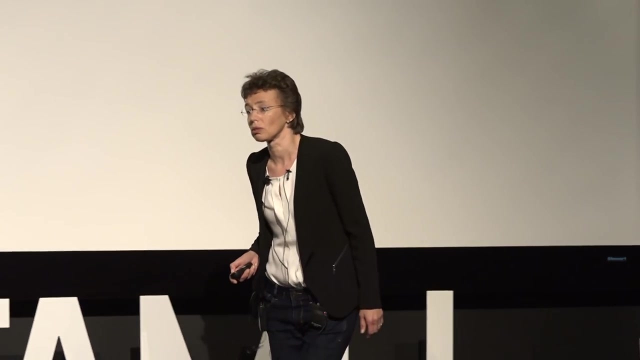 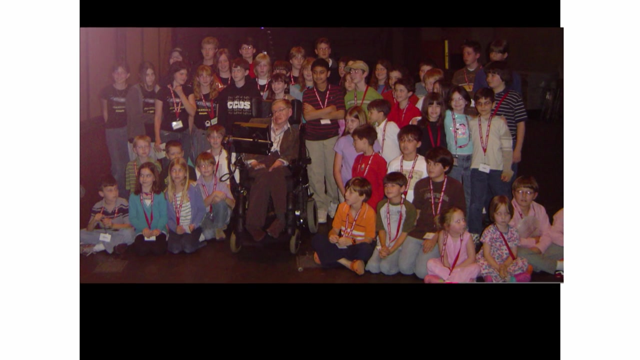 Come to our festival and ride our square wheel bike. So the very first festival finished, Thank you. It had just a dozen of hands-on demonstrations and lecture by Stephen Hawking. Thousands came. It was an amazing celebration of science from the very beginning. 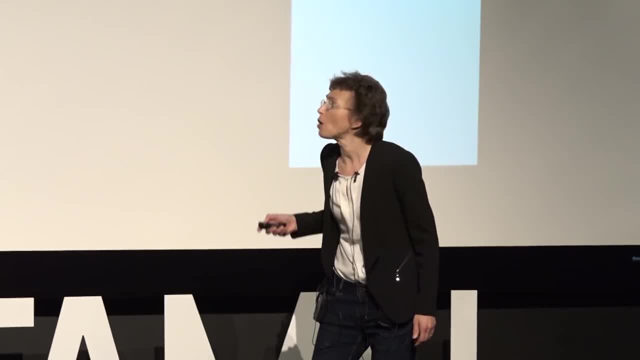 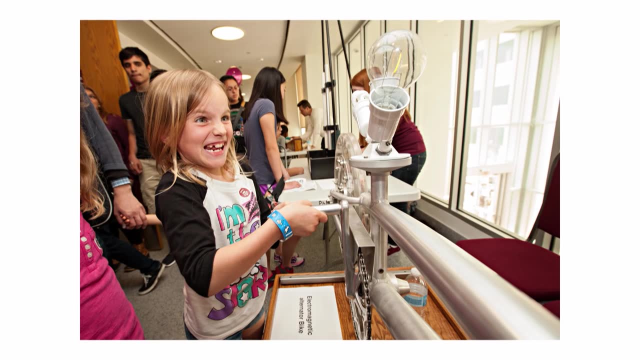 Since then it has become a tradition and annual event. Now we have hundreds of hands-on demonstrations. We bring the best speakers in the country: TED speakers, Brian Greene, Sean Carroll, Phil Plait- I can go on and on. 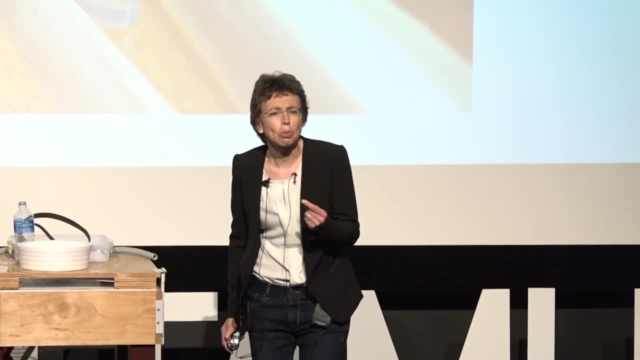 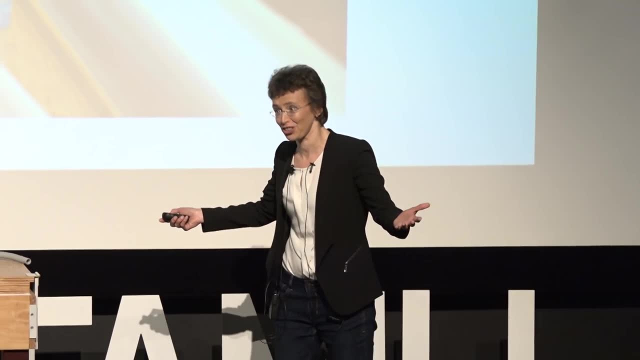 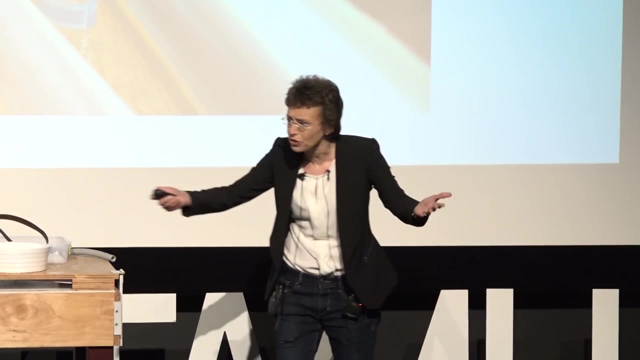 Where else? When people meet top-notch researchers, Nobel laureates, astronauts- and ask them about everything- the Large Hadron Collider, lasers, stars- I often hear that scientists cannot communicate with the public. well, But this is probably because the format is wrong. 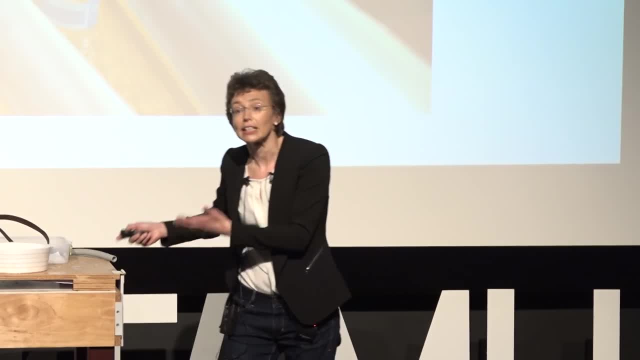 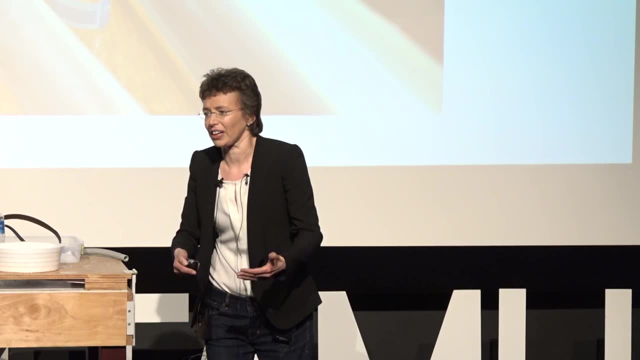 If, instead of preaching from the podium, you take your favorite hands-on demonstrations and you go outside, you go to people, then it's so much easier to start the conversation, to engage people. So many more will listen to you and appreciate your research. 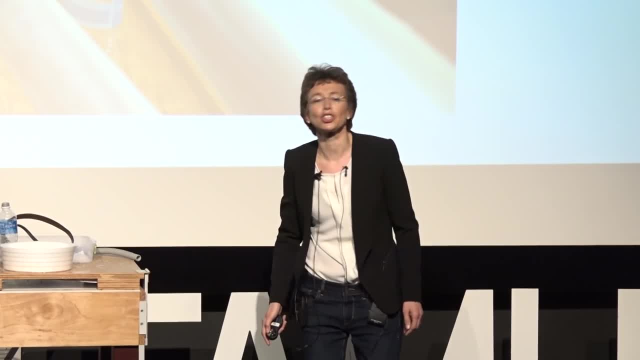 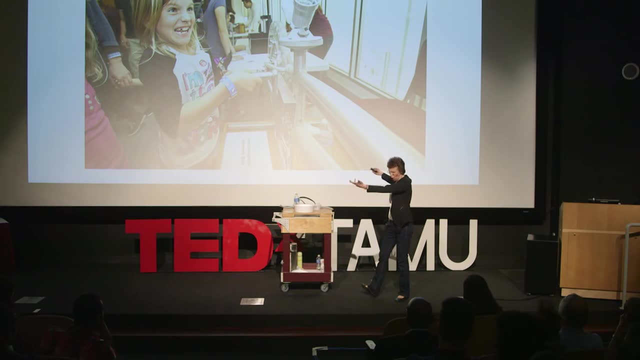 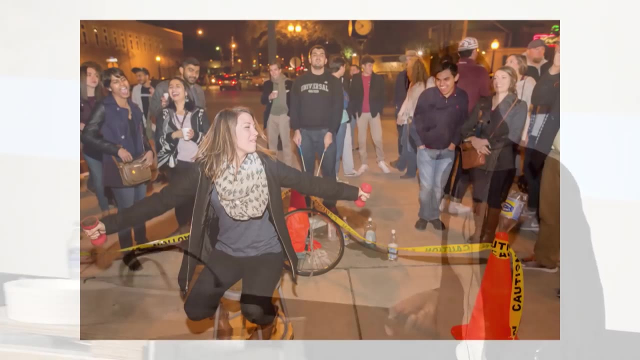 This year, for the first time, we took our hands-on demonstrations to the first Fridays in downtown. Imagine this Street: musicians, Texas food and wine and physics. We had big crowds. People were so grateful. You can take something as simple as a piece of hose from a building. 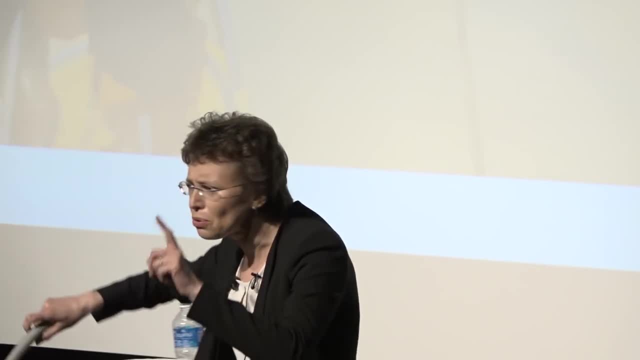 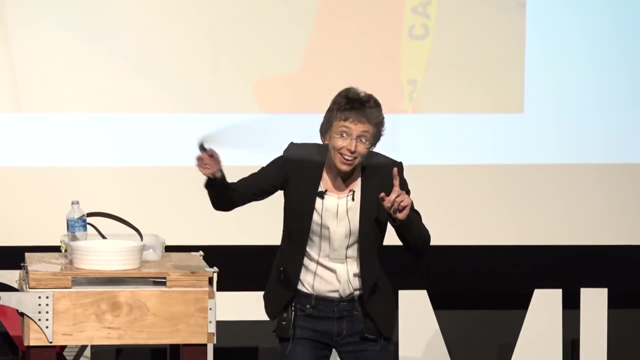 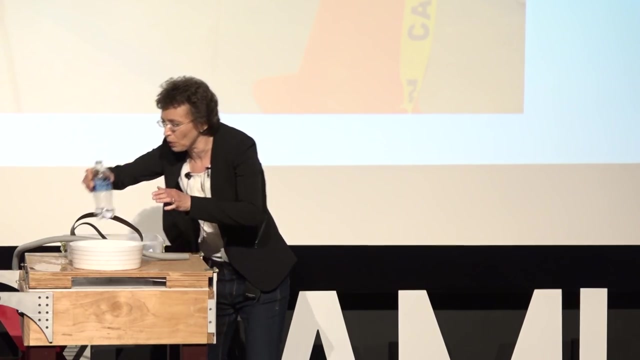 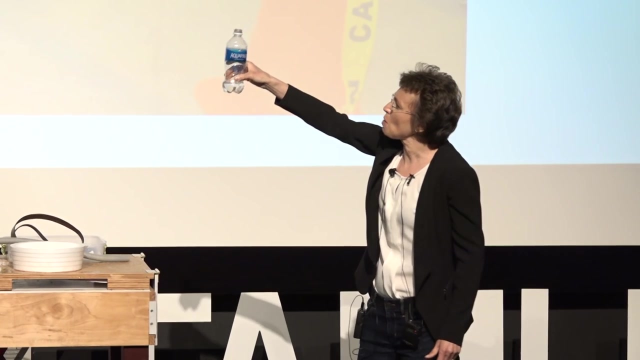 A piece of hose from your washing machine And this piece of hose will sing beautiful songs. Or you take a bottle of water and this bottle will demonstrate the magic of atmospheric pressure. You see, I have water there right Now. I put it upside down. 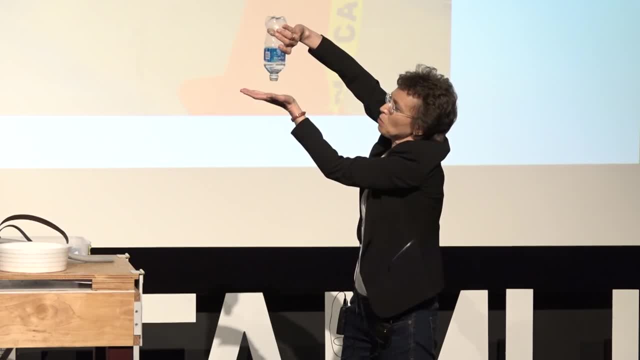 Well, water stays in No pressure inside, Atmospheric pressure outside. Difference in pressure holds water in The bottle. right Now I want water to come out. How can we do that without squeezing the bottle? I cannot squeeze the bottle, So what should we do? 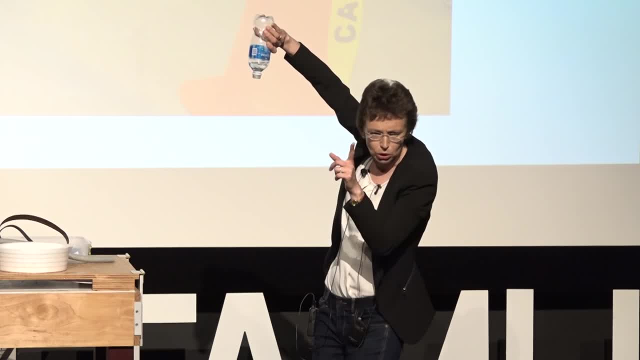 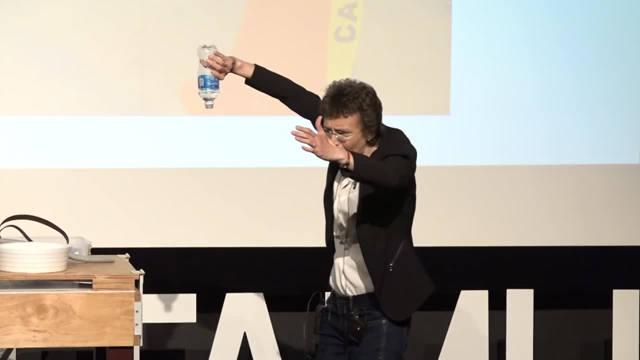 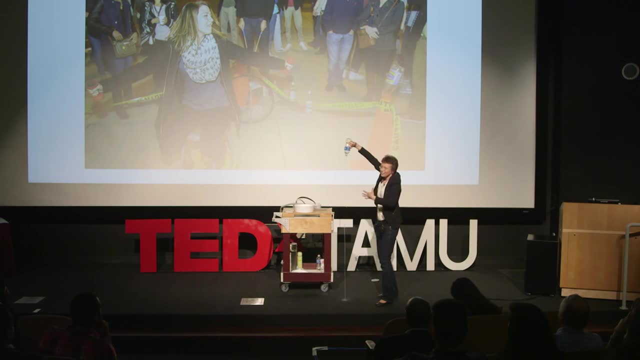 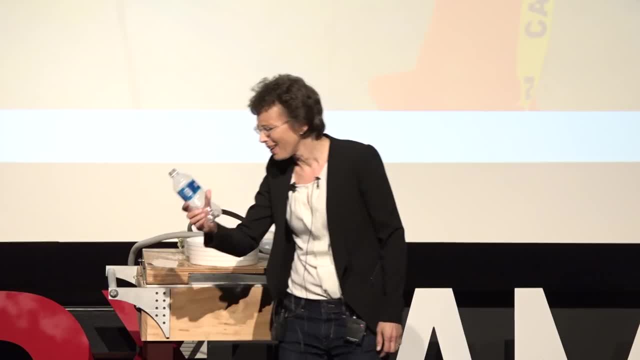 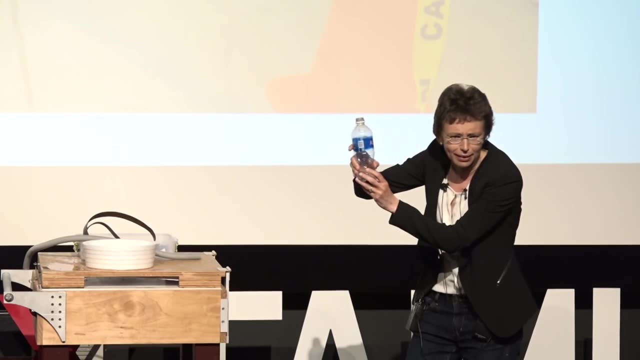 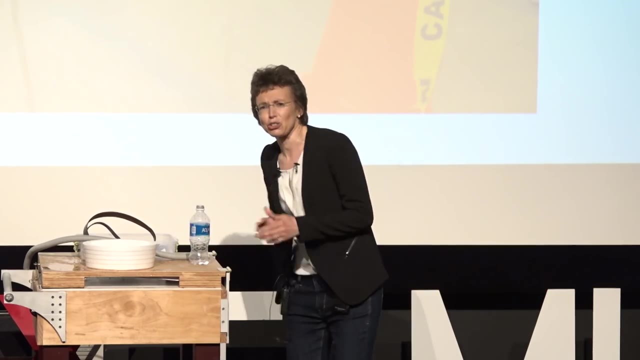 Of course I cheated. I have a tiny hole here. At first I close it with my finger, Then I opened it. I let the A in equilibrating the pressure And the story gets better. When we talk about science festivals, we always talk how important it is for the public to 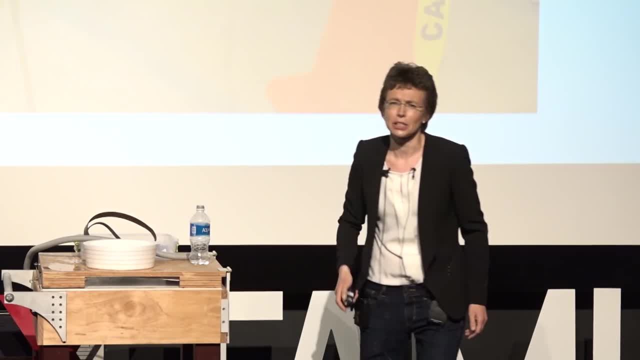 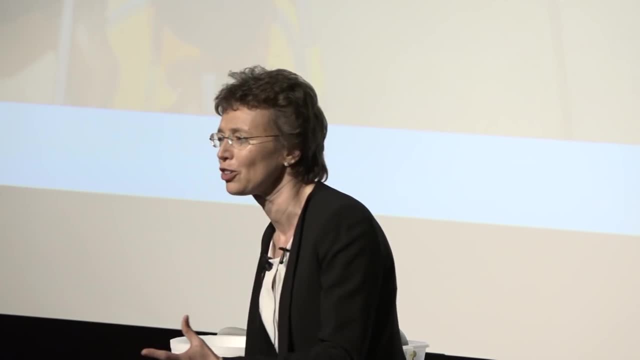 come to the festivals, we often forget how important it is for our students. The students get a unique chance to serve the community by applying their knowledge, their expertise, and this is priceless. In 2012,, we started a new program that we call DEEP. 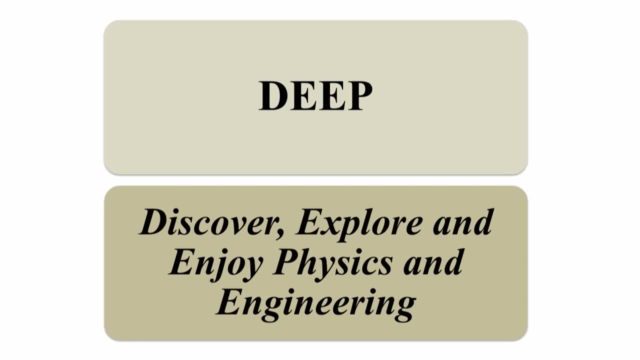 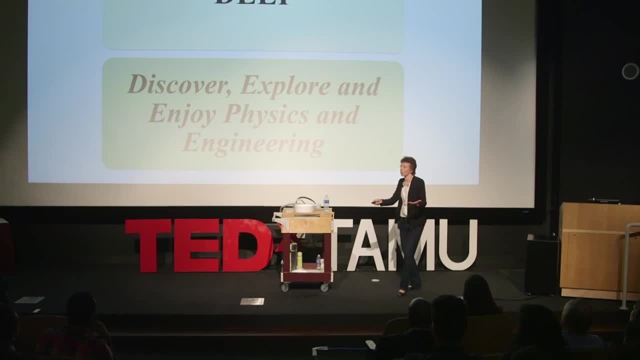 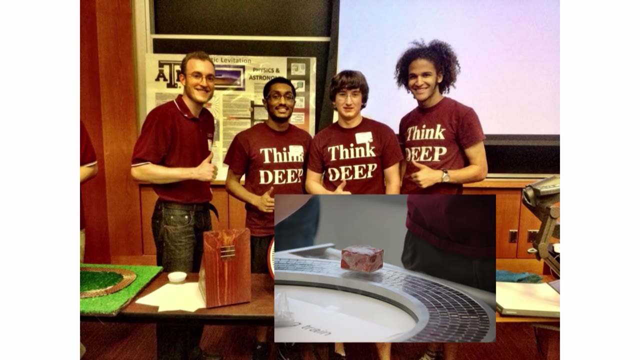 Discover, Explore and Enjoy Physics and Engineering. Our students work in teams on building new, exciting hands-on demonstrations that they share with our visitors. This team built a magnetic track with a superconducting train levitating over it. Most of these students were freshmen when they built this demo. 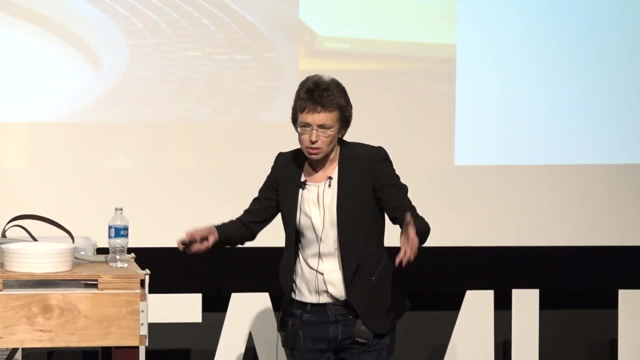 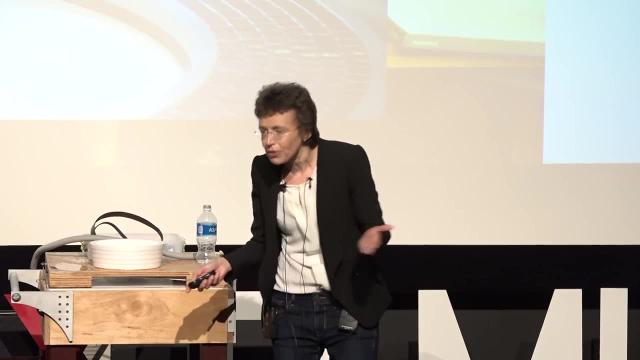 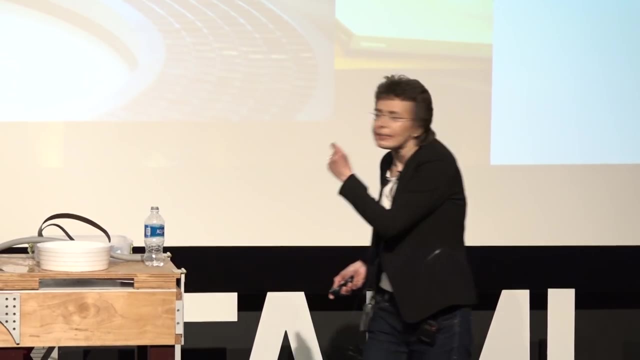 How many of you remember sitting in these large freshman classrooms and feeling that nobody cares about you, nobody even knows that you exist? These students will always feel that they achieved something important. They built a demo that will help them. It will be displayed for years. 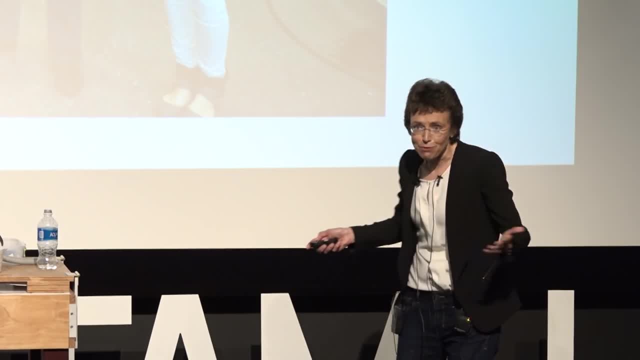 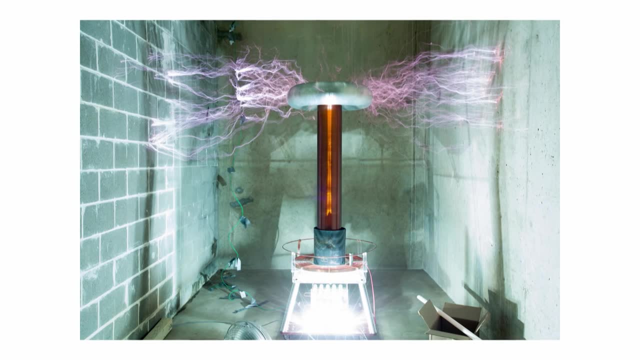 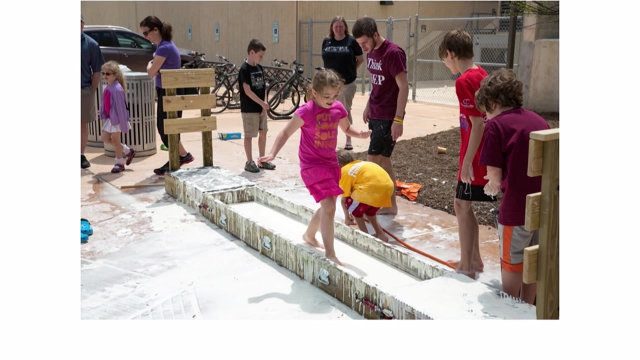 They left a legacy. Some of these demos are sophisticated and require faculty participation and, believe me, a lot of safety training, like Texas-sized Tesla coil. Some are quite simple, like a cornstarch pool. If you mix cornstarch with water, you can run on it, if you do it right. 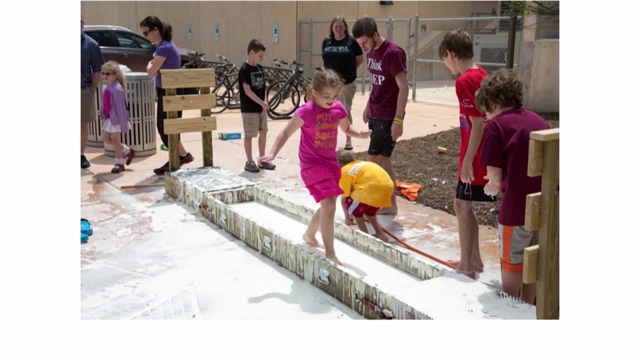 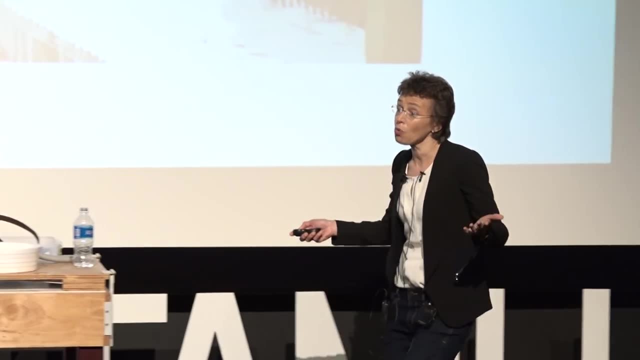 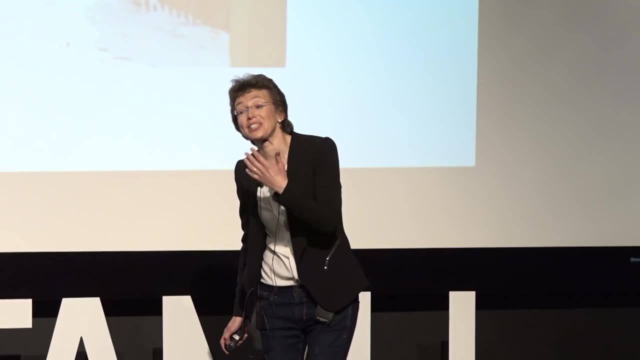 But if you stop, you sink. I remember the evening when the students put together the cornstarch pool for the first time. It was Friday. I met them and asked: how was it? The answer was the best Friday ever. The best way to understand something is to explain it. 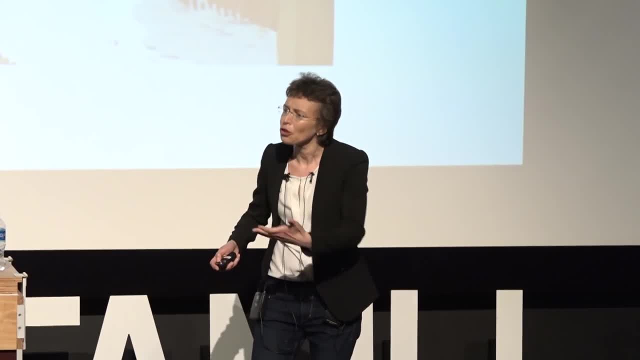 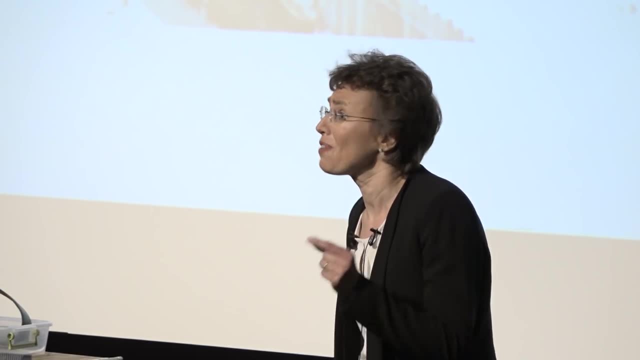 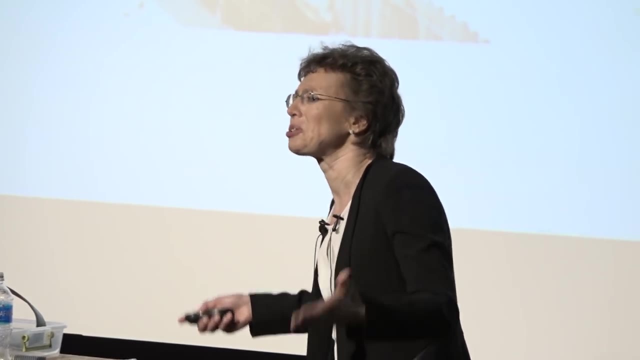 And our students get a unique teaching experience through communication with our visitors, And festival brings all of us together On the day of the festival. no one cares Are you a Nobel laureate or a freshman. Everyone works extremely hard to make the festival. 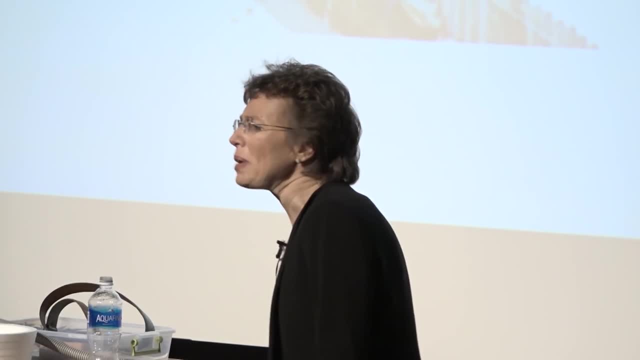 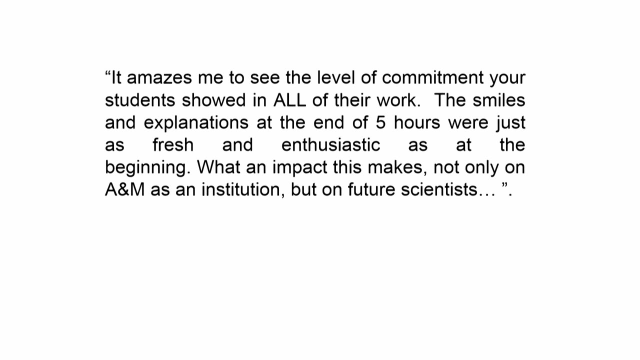 And it's an extraordinary event. We received many nice comments about the festival. I will share with you just one of them. A person wrote to us: it amazes me to see the level of commitment your students showed in all of their work. 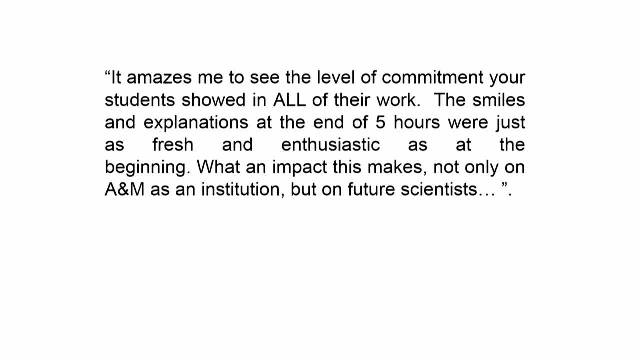 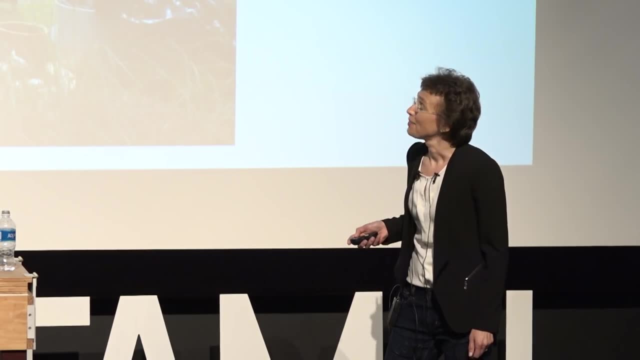 The smiles and explanations at the end of five hours were just as fresh and enthusiastic as at the beginning. What an impact this makes, not only on A&M as an institution, but on future scientists. Enough of that, Thank you. The other person said this is so much for so many people.